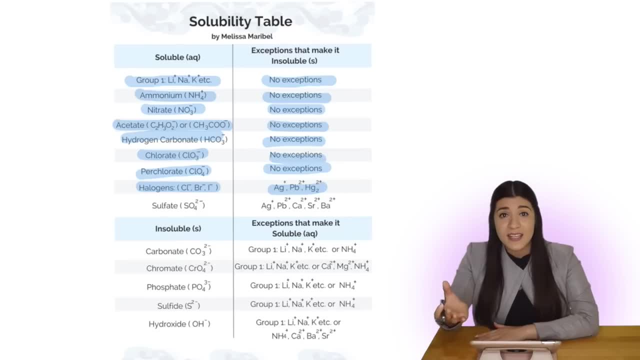 that makes it insoluble, meaning it's a solid. But if those metals were not attached to a halogen, then we know it would be aqueous, making it soluble. The last one on this column is sulfate, And then we have a lot of exceptions to our rule in this case. 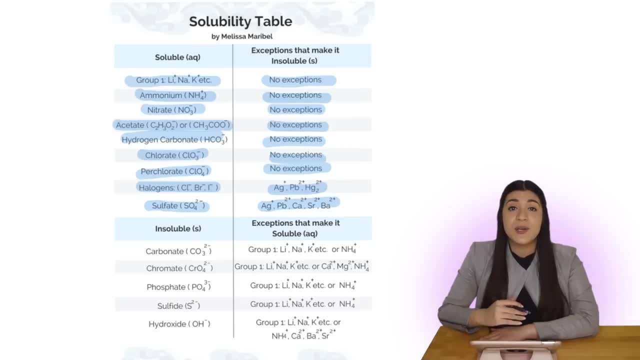 All of these metals, when they're attached to sulfate, means it's going to be insoluble or a solid. Next we're going to move on to the bottom portion of our solubility table, And all of these are normally insoluble, with a few exceptions. So let's look at carbonate. 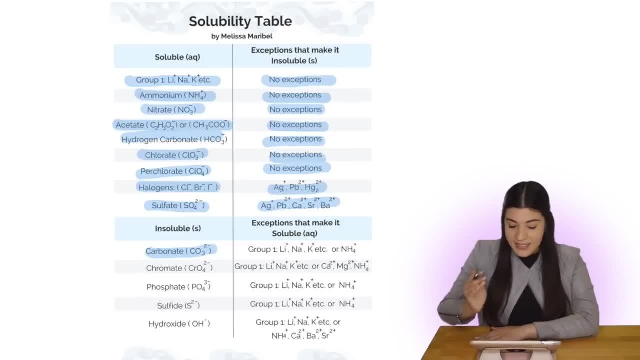 That's typically a solid. but we're going to have exceptions to that rule that make it soluble or make it aqueous. So if we have anything in group one or ammonium attached to carbonate, that would mean it's soluble, meaning it's aqueous. But if we don't have 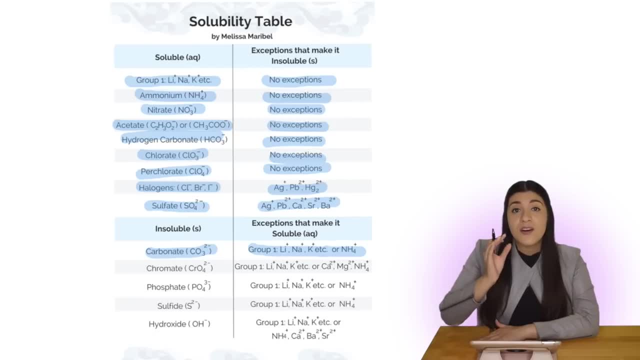 any exceptions to that rule, then we know that carbonate is typically a solid. Let's move on. So let's look at chromate, Same sort of concept. here We're going to have exceptions to that rule. So if it's group one- metals or calcium- 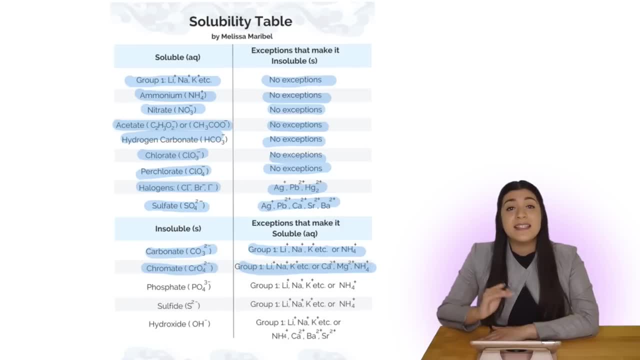 magnesium or ammonium attached to chromate, then that means it's aqueous or soluble, And then phosphate. similar concept here: Whenever we have group one- metals and ammonium- attached to phosphate, then that means it's aqueous again, And you're going to see this trend over and over. 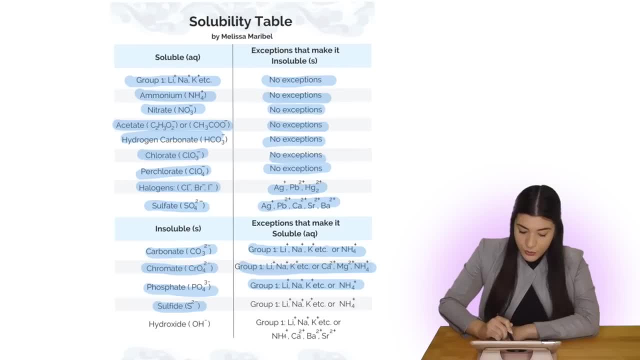 Now we have sulfide and whenever that's attached to group one- metals or ammonium- then we know that's going to be aqueous. but if it's not attached to any of those exceptions to our rule, it's still aqueous. So if it's aqueous then it's not going to be aqueous. 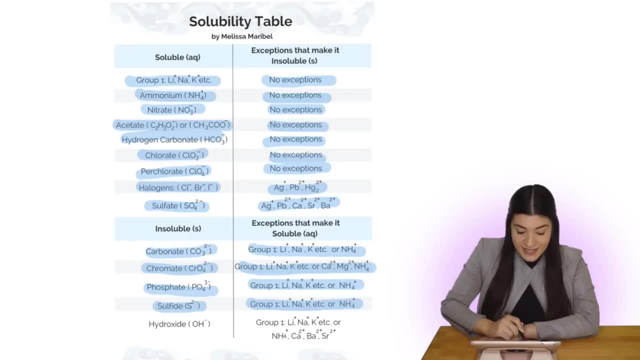 then we know that it's typically a solid And then, lastly, hydroxide. whenever it's attached to group one metals, or ammonium or any of these other metals, then we know it's aqueous. but if it doesn't have that exception, 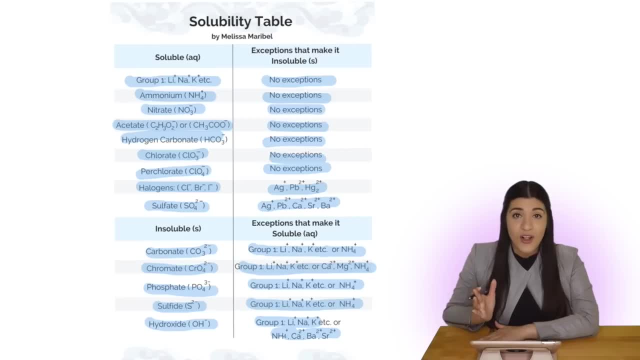 or that metal attached to it, then we know it's a solid. All right, so now that you have a better understanding of a solubility table, let's try to predict the solubility of different compounds. So in our first example here, 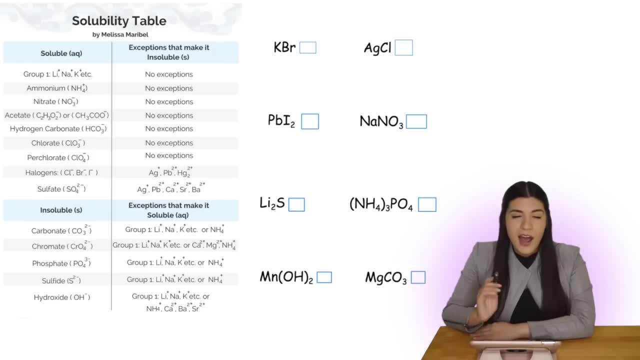 we have potassium bromide. Now where I usually start is I start with the last element attached to that compound. So I'm gonna start off with bromine. Now, if I were to look at that, I'm gonna go back and identify. 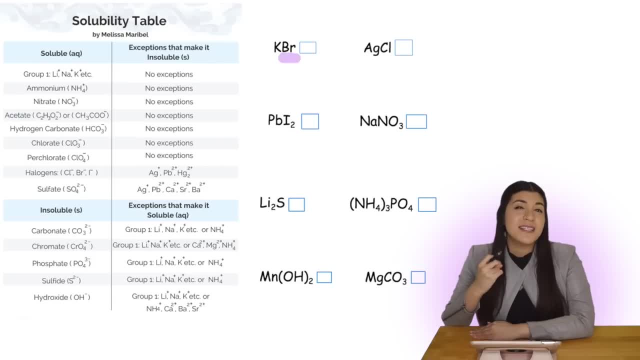 where is bromine on my solubility table and what exceptions are there to that rule? Does this have any exceptions? So bromine is a type of halogen, So here we have. it's typically soluble, with the exception of silver, lead or mercury. 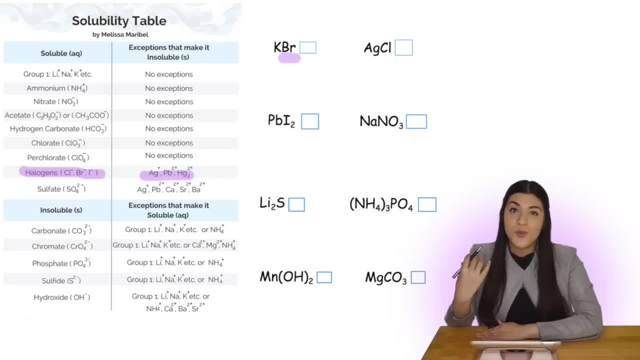 but potassium or K falls under group one, which we know, okay, that those are always soluble. So right then, and there we know that this is soluble, So this must mean that it's aqueous. Let's move on to our other example. 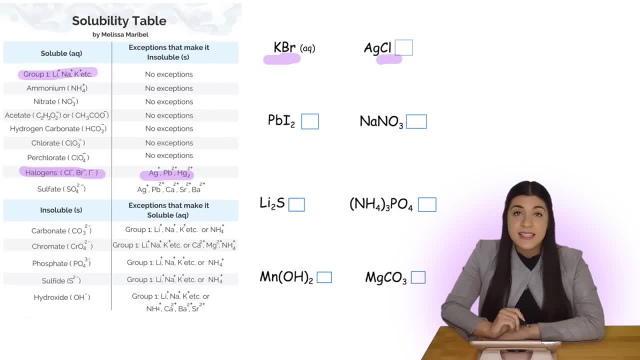 Now I'll do the same thing. I'm gonna look at the end and I see that it's chlorine. Once again, that's our halogen. And then does this fall under any of the exceptions? Yes, it does, because silver is one of those exceptions. 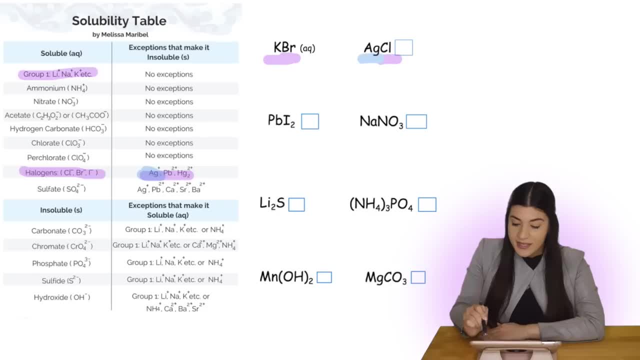 to our rule making it insoluble. so we know that this entire compound is insoluble, or we can also state that this is then a solid. Now let's look at iodine here. Oh, we're starting with the second element within the compound. 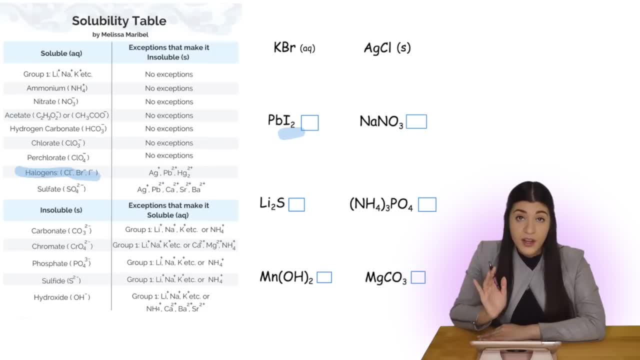 And I know once again that's a halogen. Does lead fall under one of our other options? Does calcium fall under one of our other options? Does sodium fall under one of our other options? Does copper as much as you think it should be? 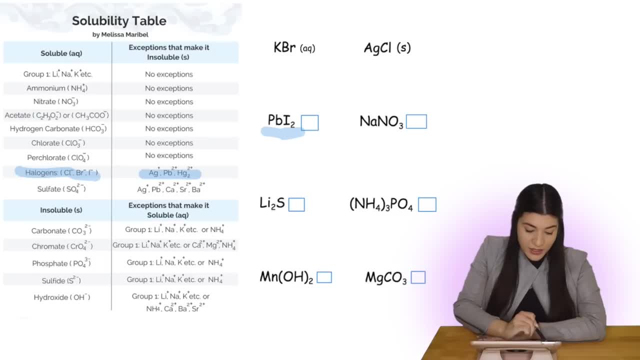 Does sodium fall under one of our other options, our exceptions? yes, it does so, automatically. we know that this is going to be a solid. now let's look at nitrate. nitrate has no exceptions, so it's always soluble, no matter what. therefore, we know it's aqueous. moving on to sulfide, so sulfide is typically insoluble, with the exception of any. 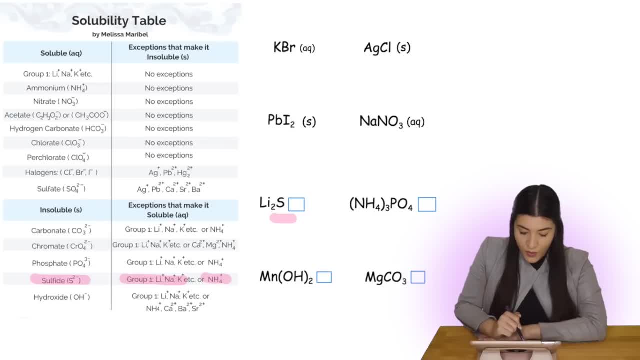 metals in group one, or ammonium, so lithium is in group one. it does fall under that exception, so we know this compound is then soluble or aqueous. next we have phosphate, so po4 is typically insoluble. however, with the exception of- once again, is it in group one. those metals.